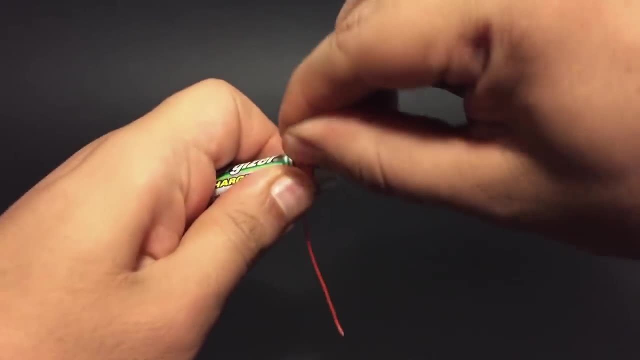 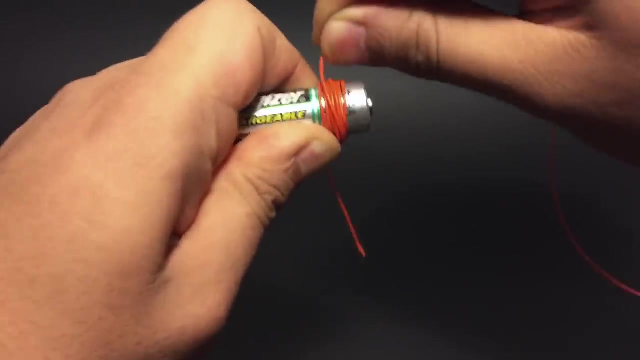 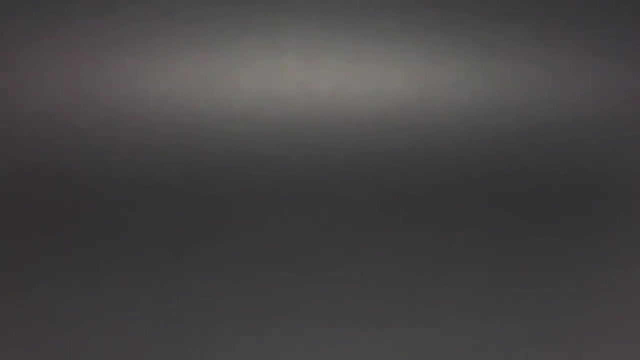 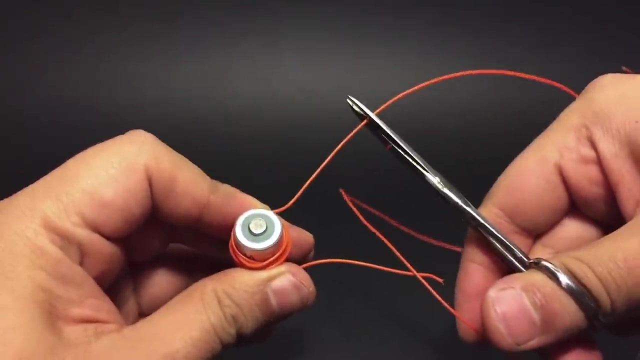 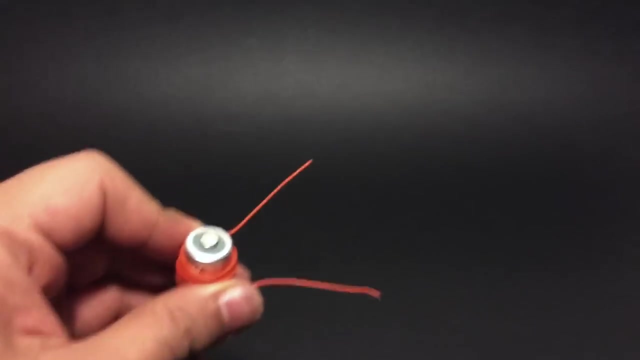 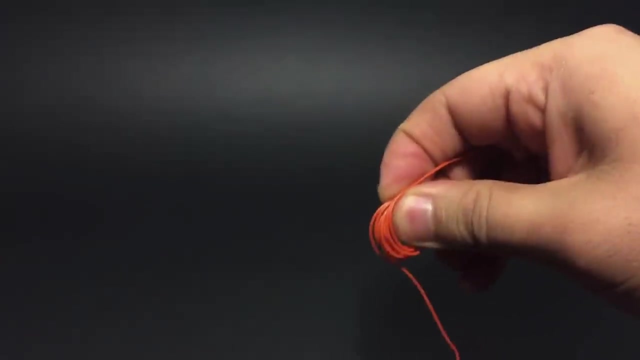 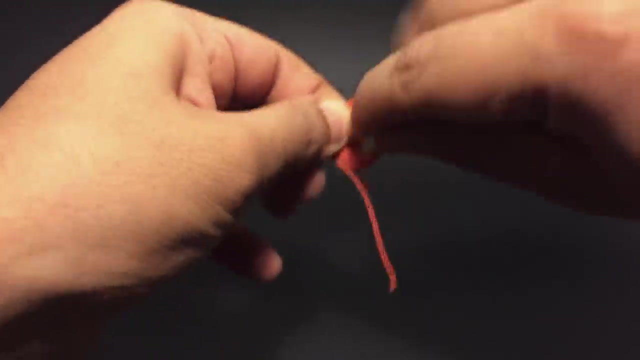 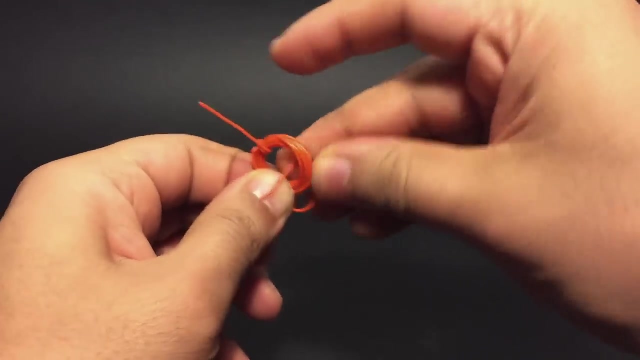 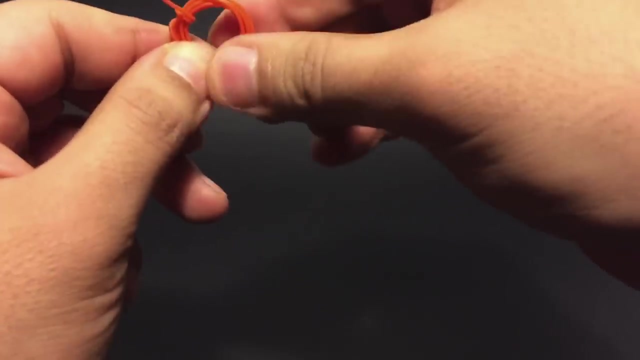 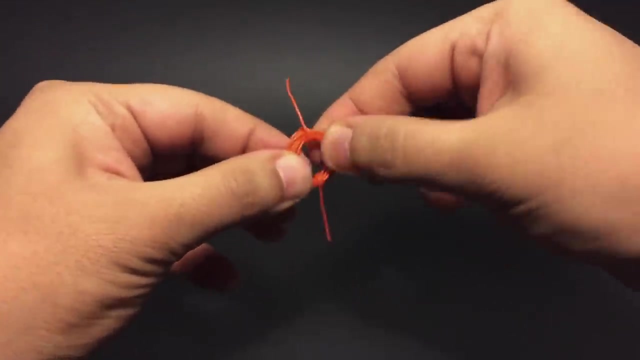 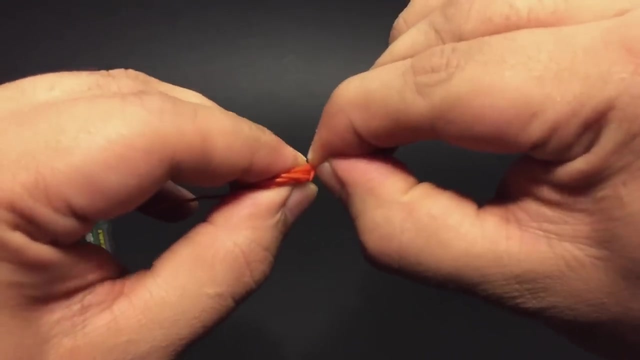 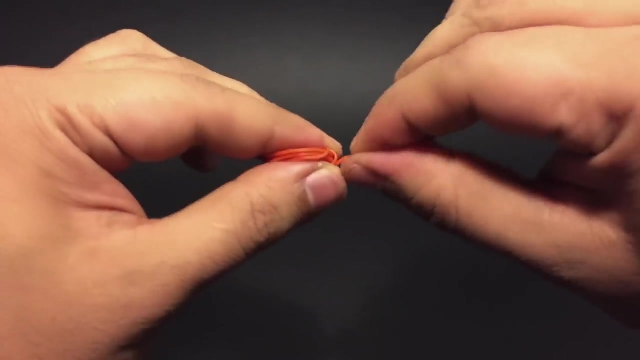 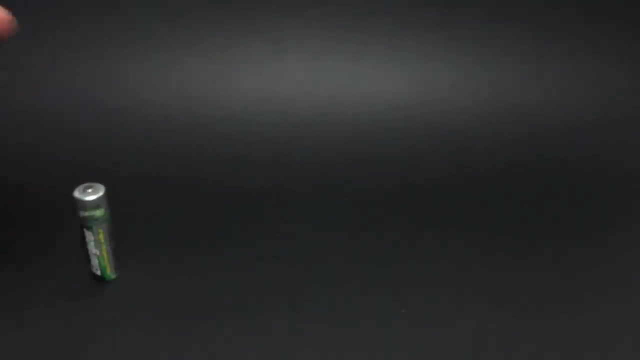 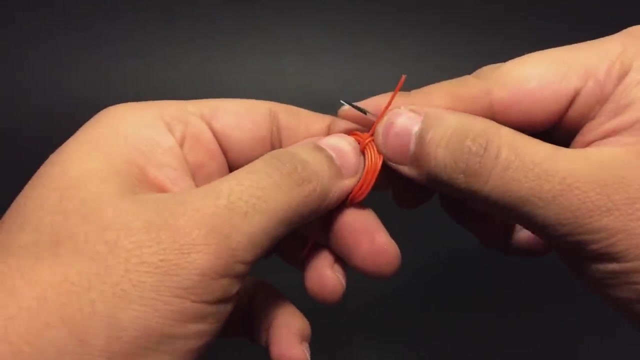 ten times. We need two inches on each end. Remove the coil from battery and wrap the ends around the coil two times. Step two, As a show Com全. Remove the insulation and be careful not to damage the wire. Okay, Bye, bye. 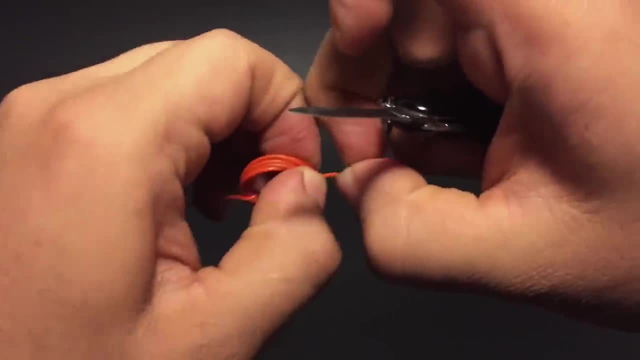 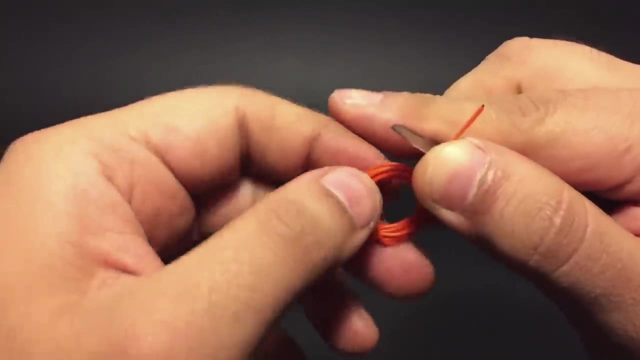 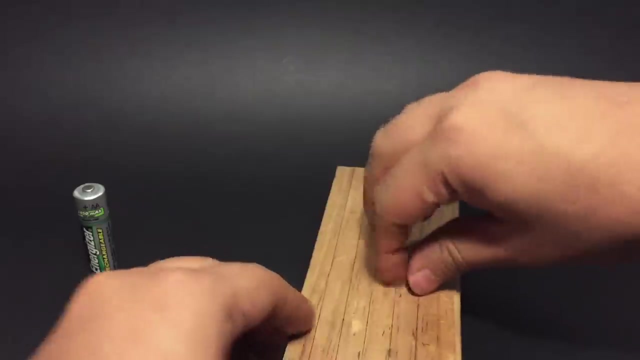 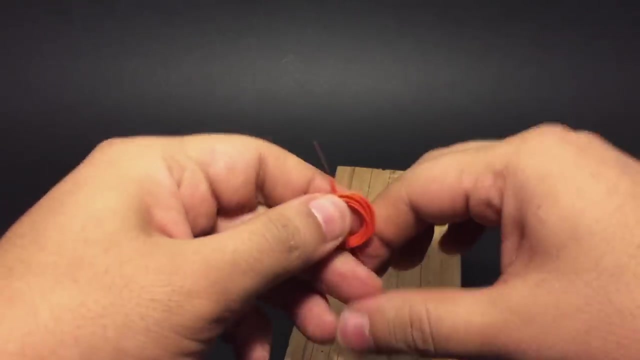 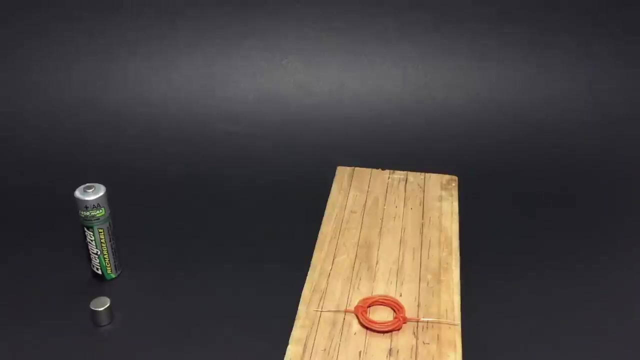 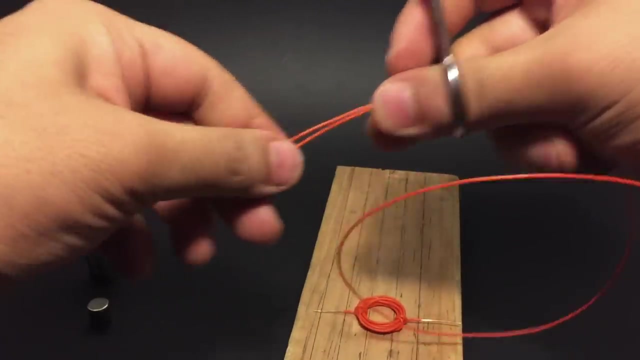 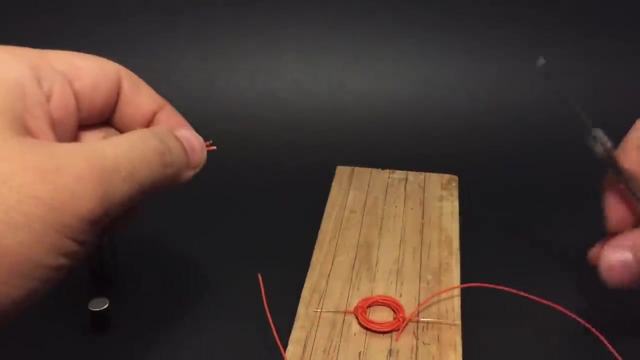 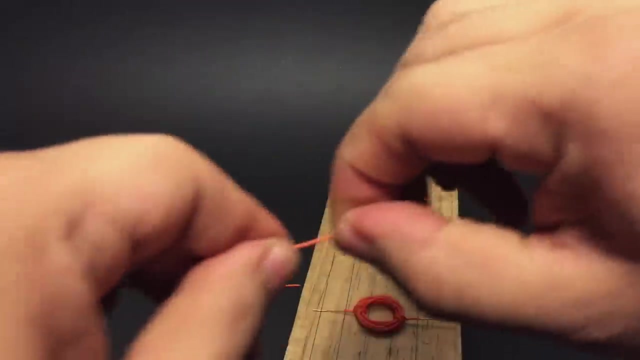 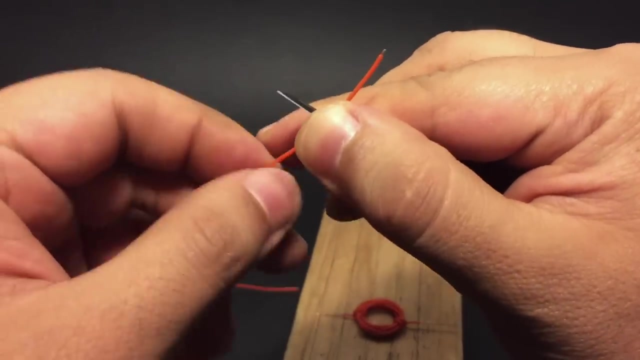 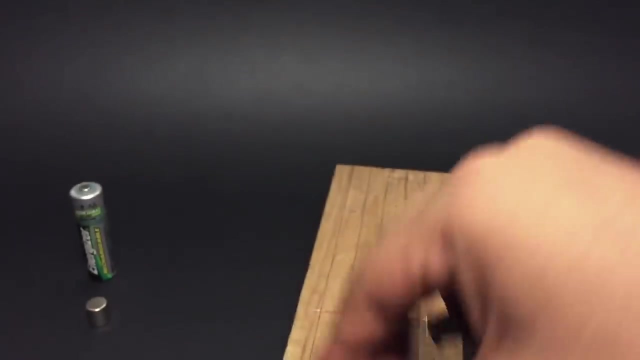 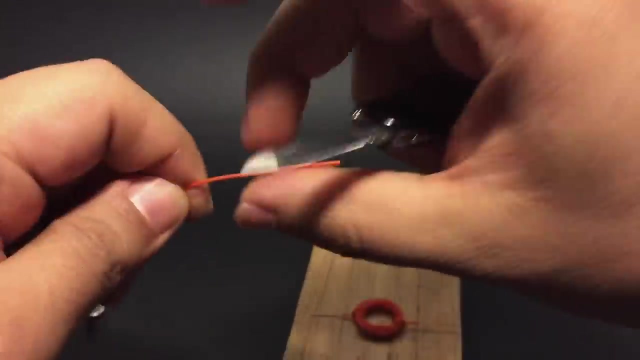 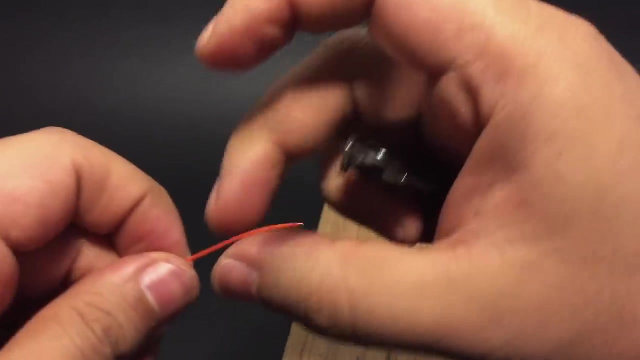 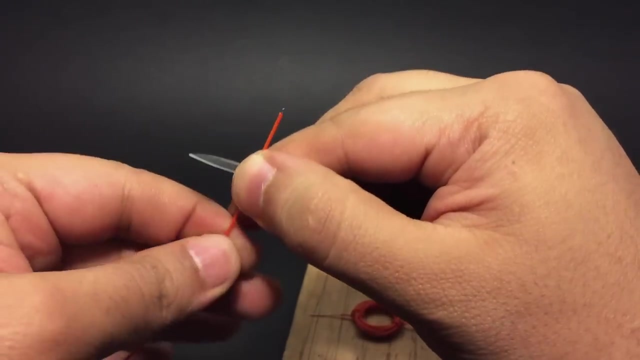 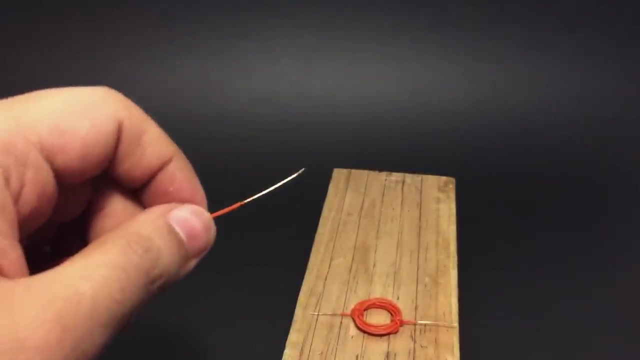 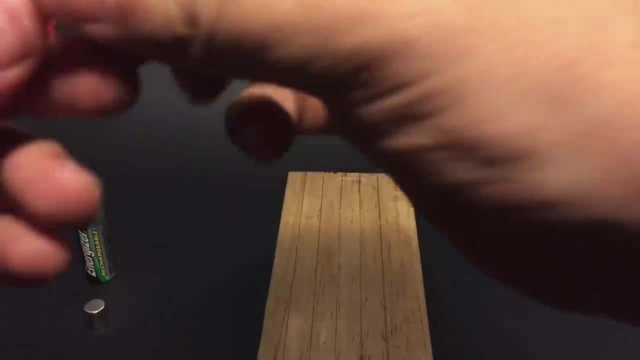 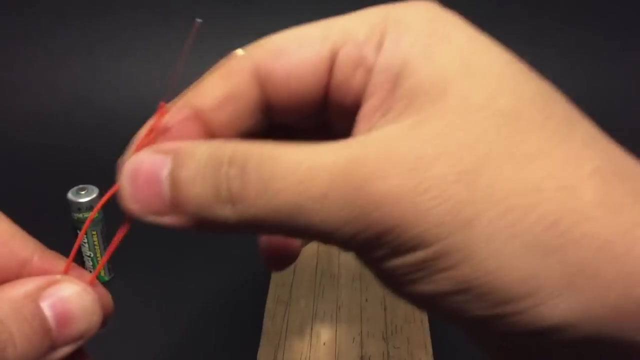 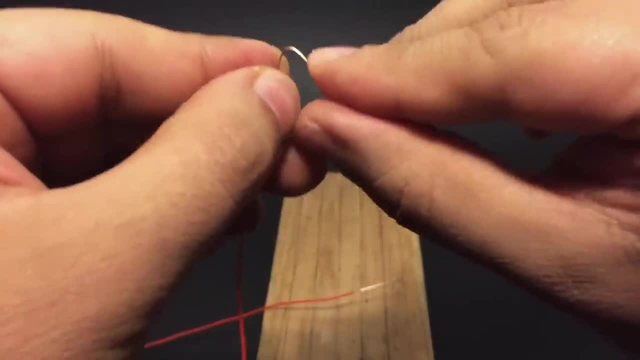 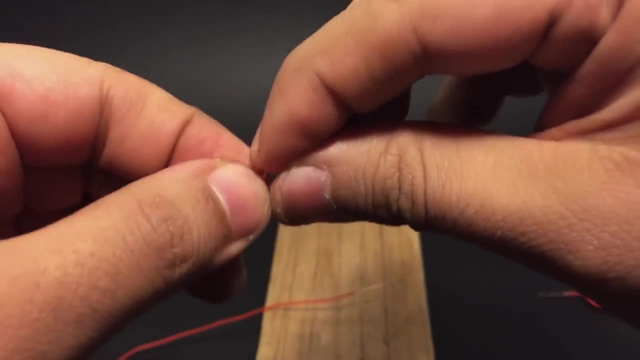 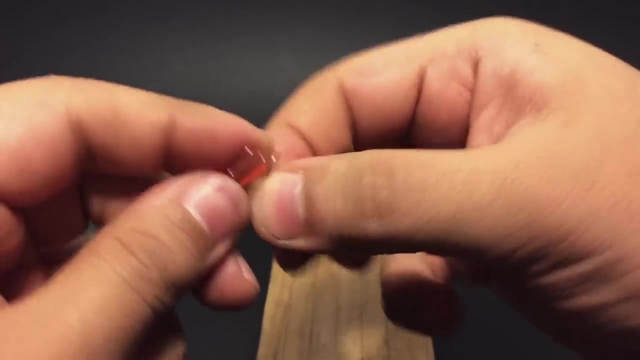 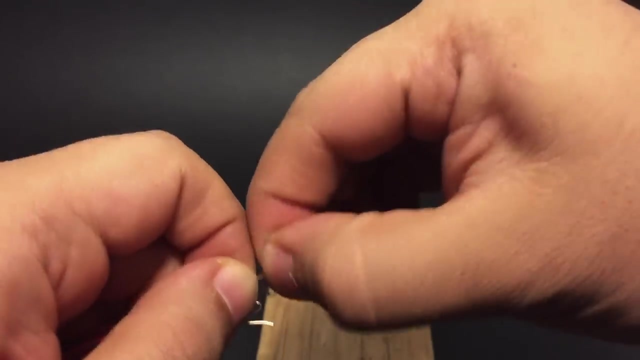 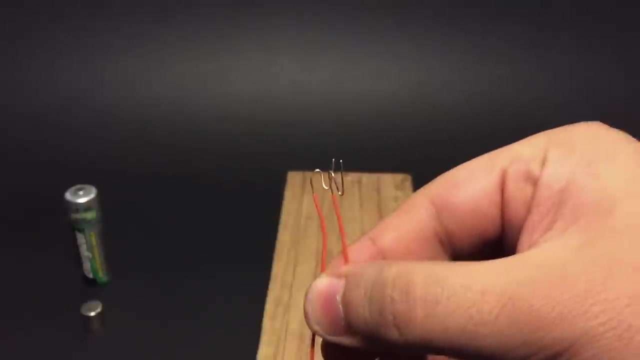 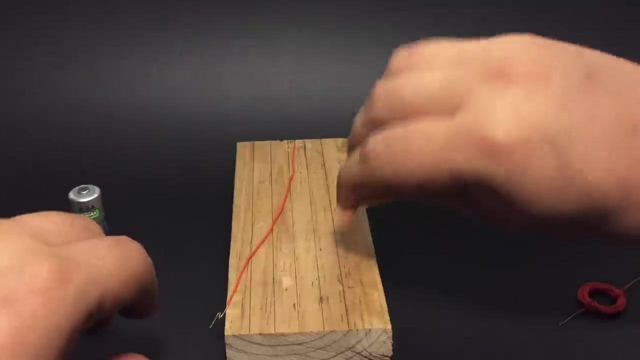 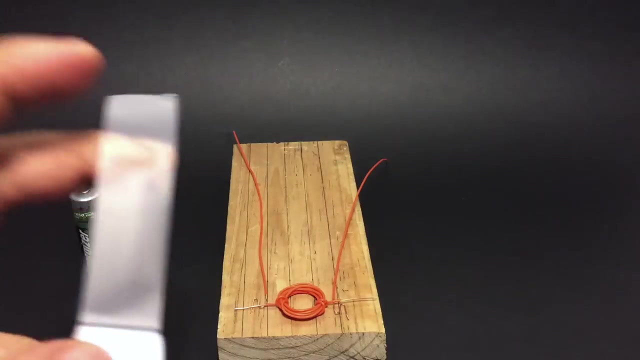 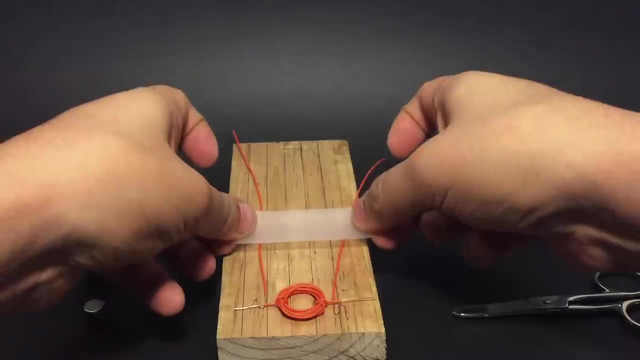 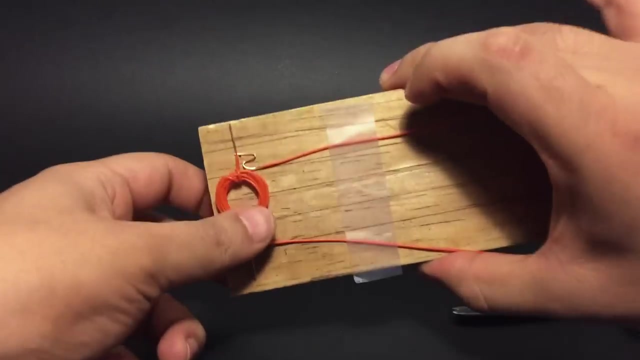 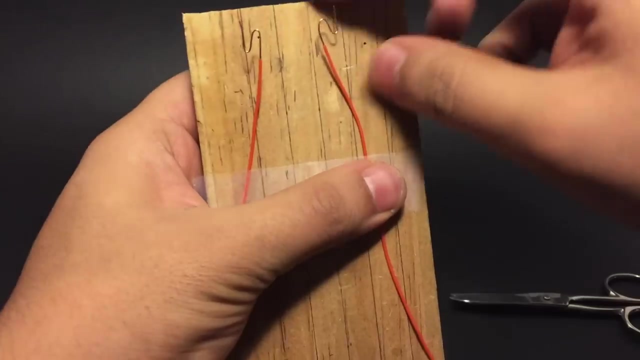 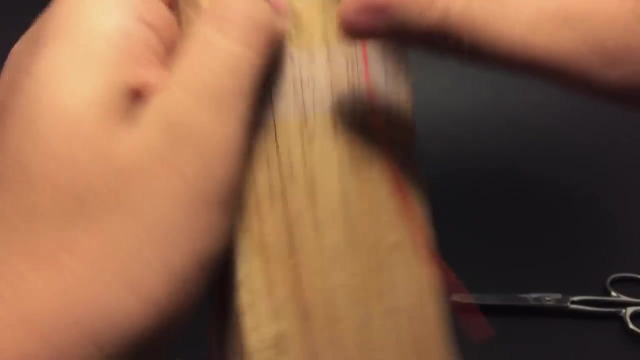 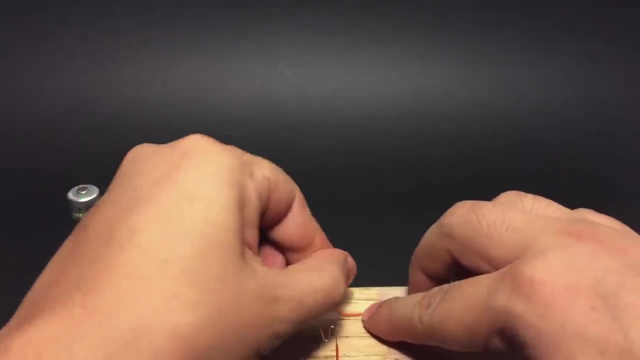 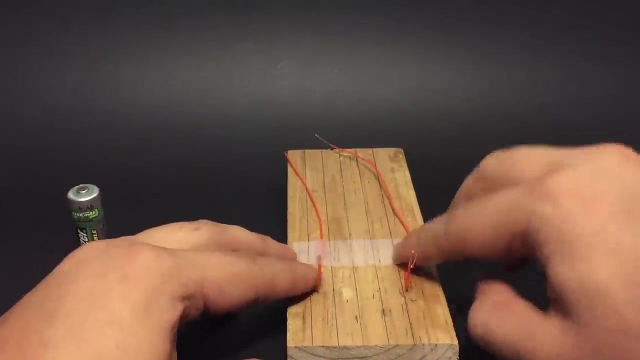 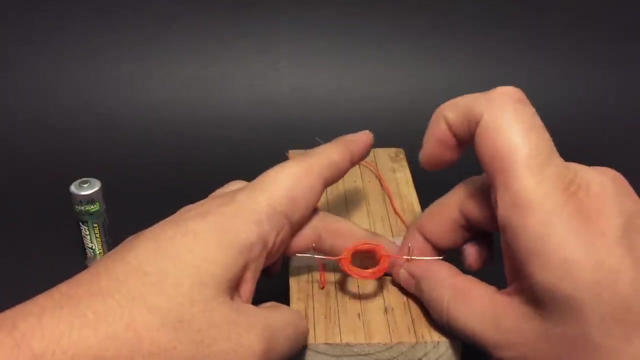 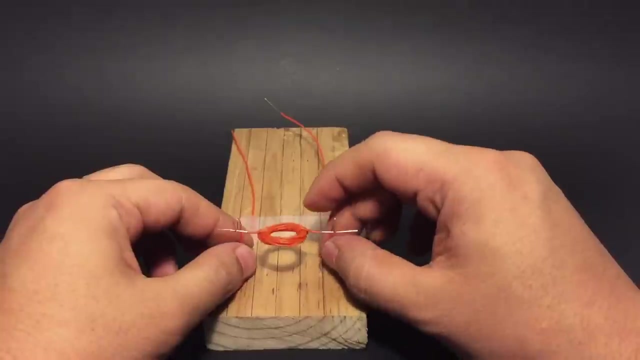 For each wire bend and form an S-shape. Step 3: Now fix the wires to wooden block using tape. For each wire bend and form an S-shape. Each wire bends about 90 degrees. You may need to make some adjustments. 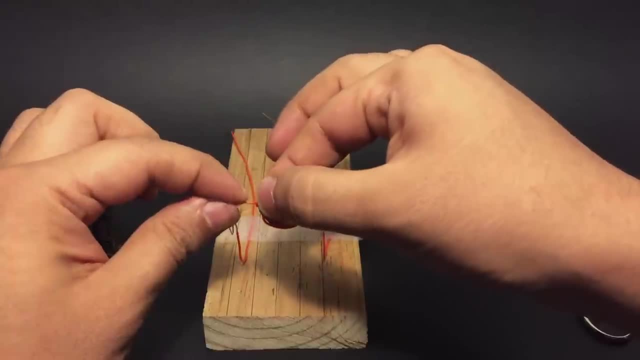 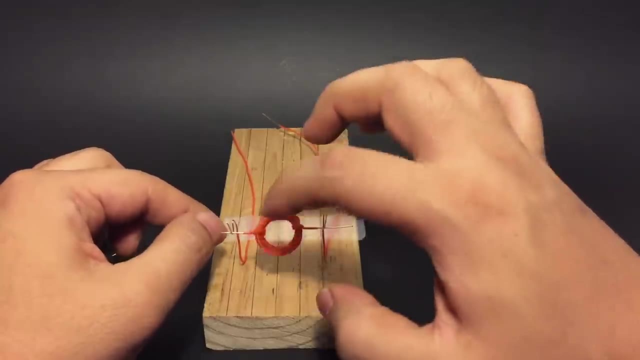 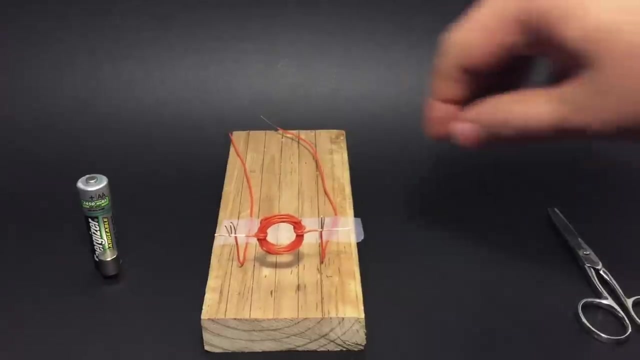 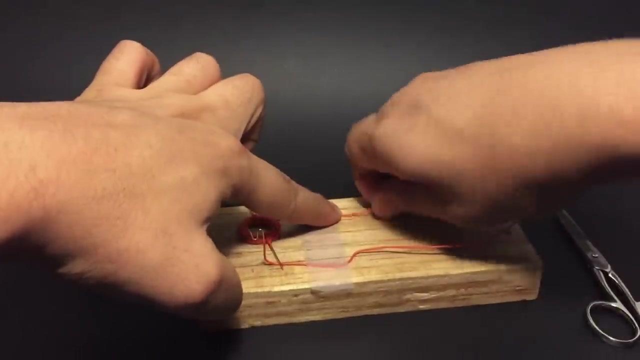 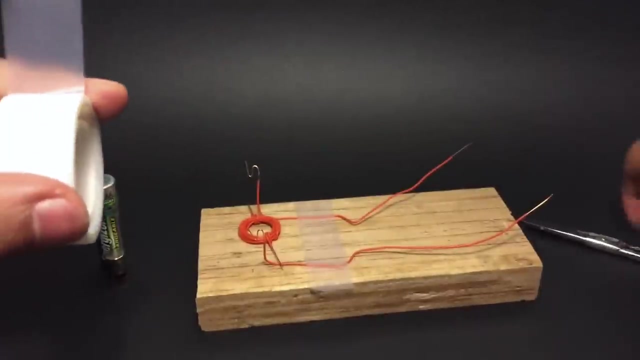 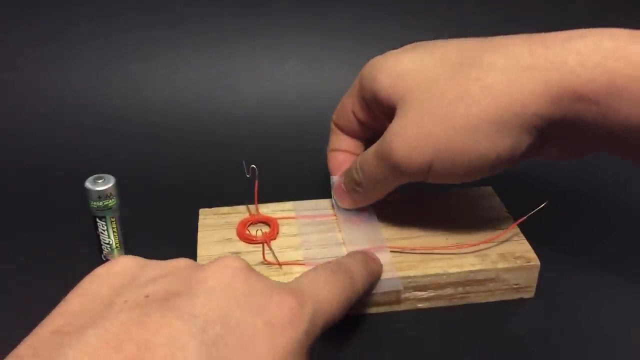 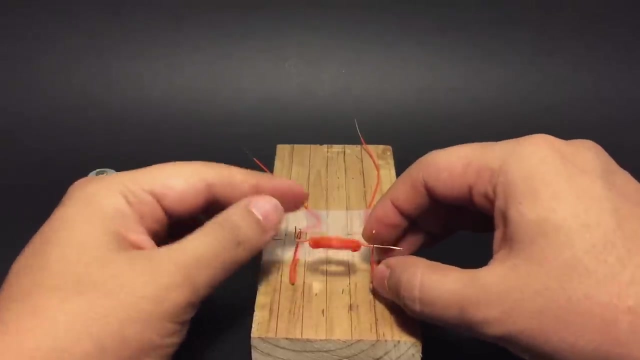 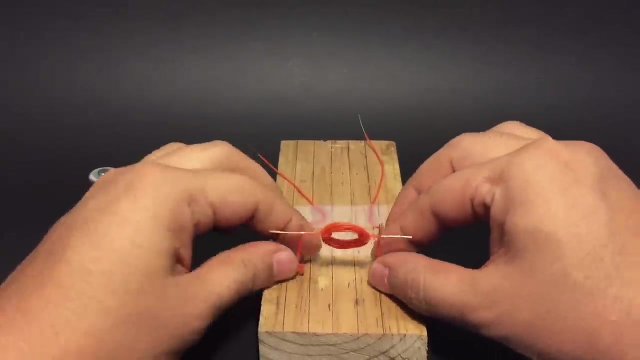 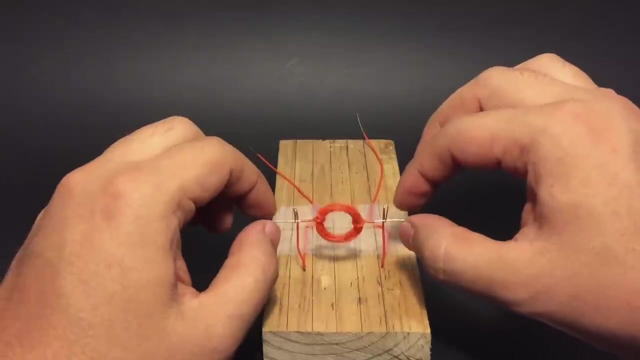 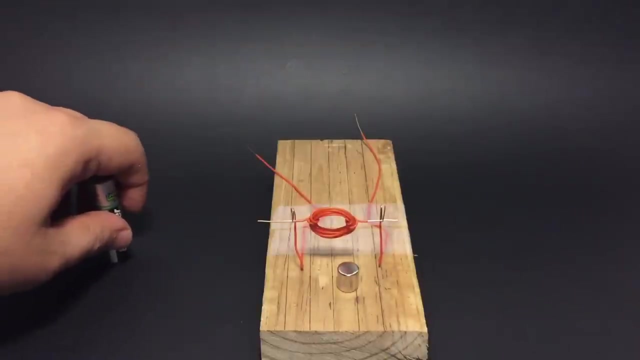 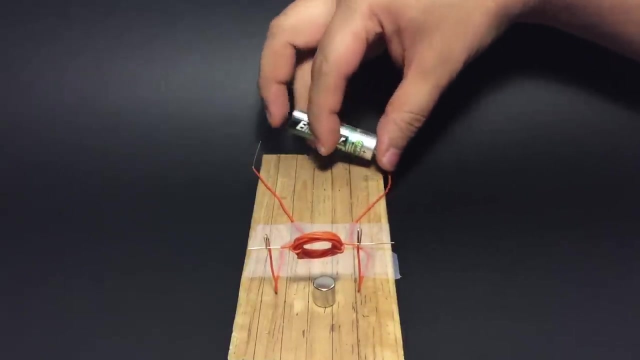 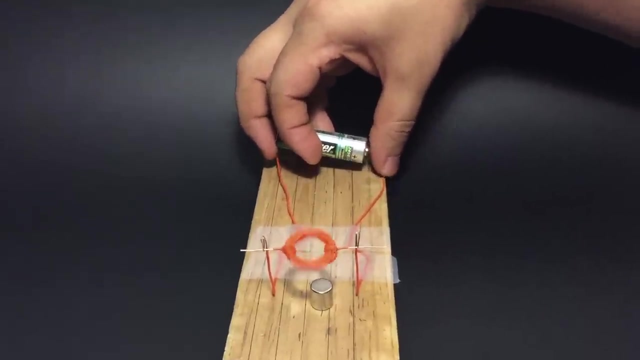 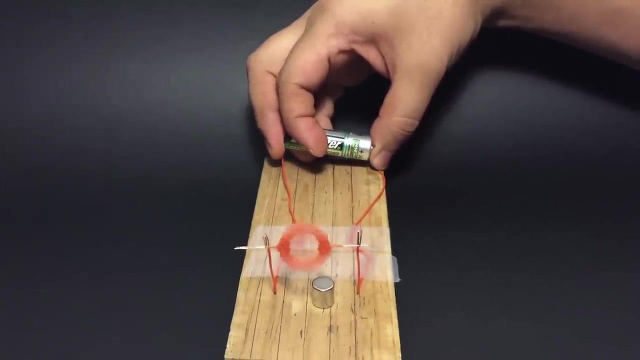 Make sure the coil is centered and balanced. Make sure the tip goes in the right direction. Make sure the coil is centered and balanced. Step 4, put the magnet under the coil and connect the battery. We did it. Hope you've enjoyed it.